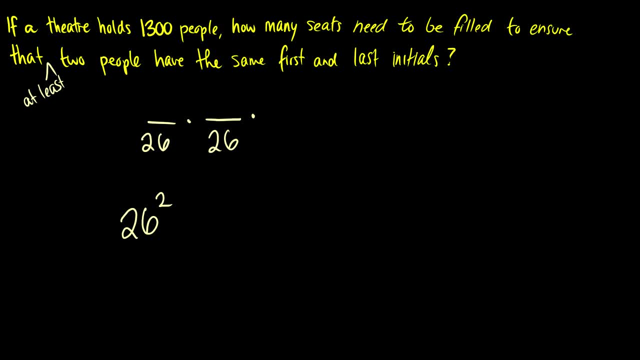 So there's 26 squared ways to make first and last initials. So that means if we have 26 squared people, then everyone could fill up all those possible sets of initials, Which means if we add one to that, we're guaranteed that somebody has the same first and last initial as somebody else. 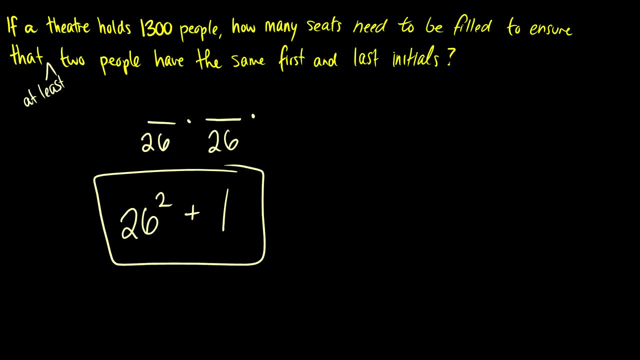 So here is our solution: 26 squared plus 1.. And you can see that this theater holding 1,300 people, completely irrelevant to the question, That is there to test to see if you know what you're talking about and if you know how this principle works. 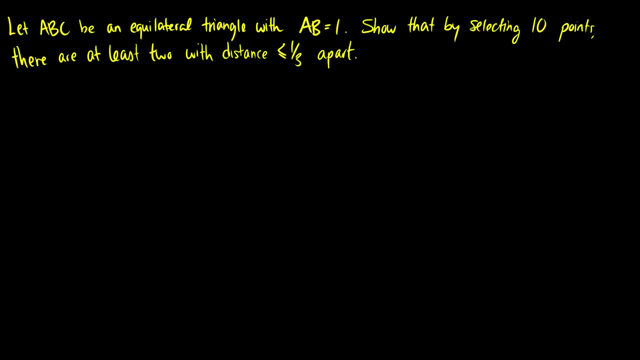 Okay, second question, a little bit trickier. I'm going to let ABC be an equilateral triangle, with AB equals to 1.. So let's draw this first. So equilateral triangle: We have A here, we have B here, we have C here. 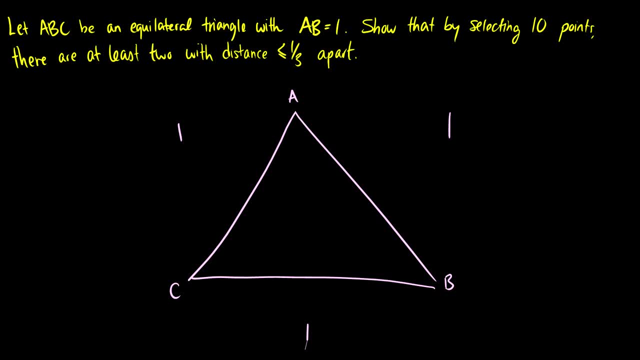 These all have lengths of 1.. Okay, And I want to show that by selecting 10 points, there's at least 2 with distance less than or equal to a third apart. Okay, so I'm targeting this number here, this less than or equal to one third. 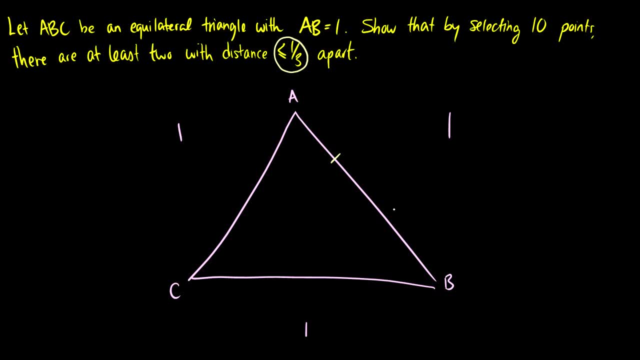 So what I want to do is I want to split up these sides into distances. So I can do this, So I just break each one up into three parts. So all of these are now one third in length. Okay, And now this is an equilateral triangle. 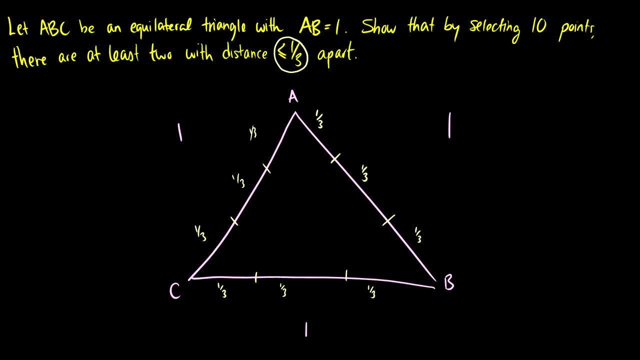 So we know, if we have two edges that are one third, then our third edge is also going to be one third, So we can make a bunch of mini triangles like this. So we have a third And this edge, we have a third in this edge. I know these supposed to be equilateral. my drawing is definitely not to scale. 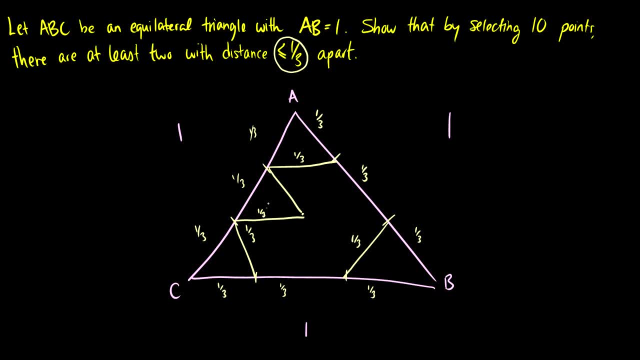 So we're going to get one third edges here, And these are all going to be one third. I will stop labeling them now, though, So these are all thirds here. So now we have- let's count how many triangles we have. we have 1,, 2,, 3,, 4,, 5,, 6,, 7,, 8, 9 triangles, and we have 10 points. 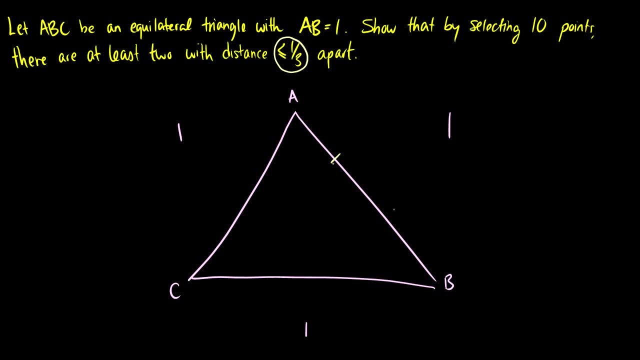 So what I want to do is I want to split up these sides into distances. So I'm going to make a triangle of 1 third so I can do this. So I just break each one up into three parts. So all of these are now 1 third in length. 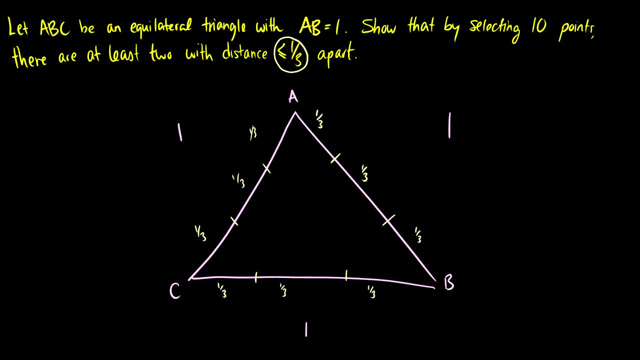 Okay, And now this is an equilateral triangle. So we know, if we have two edges that are 1 third, then our third edge is also going to be 1 third. So we can make a bunch of mini triangles like this. So we have a third. 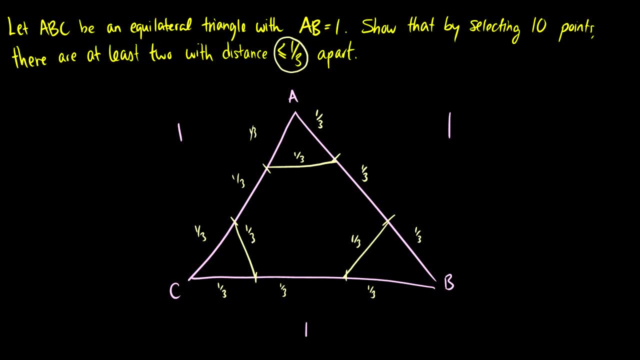 We have a third in this edge. We have a third in this edge. I know these are supposed to be equilateral. My drawing is definitely not to scale, So we're going to get 1 third edges here And these are all going to be 1 third. 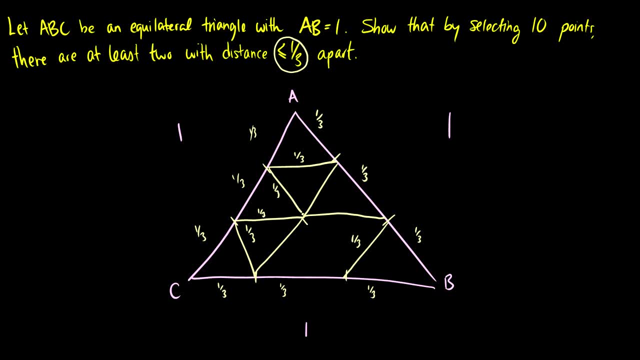 I will stop labeling them now, though. So these are all thirds here. So now we have. let's count how many triangles we have. We have 1,, 2,, 3,, 4,, 5,, 6,, 7,, 8,, 9 triangles. 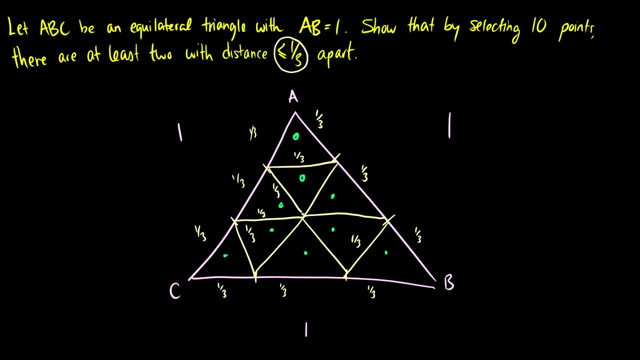 And we have 10 points. So if we put a point in each triangle, then when we put that 10th point in, what's going to happen is we're going to end up with two points in the same triangle, And we know that the points at most in a triangle can be 1 third apart. 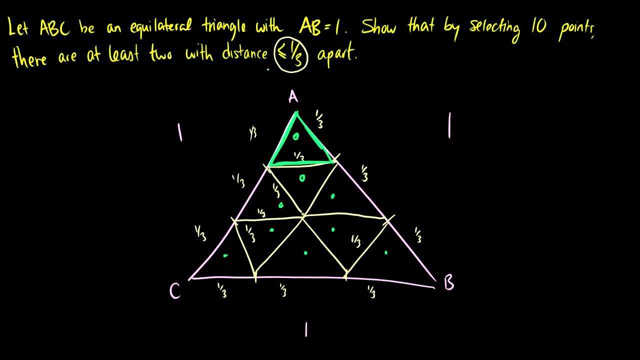 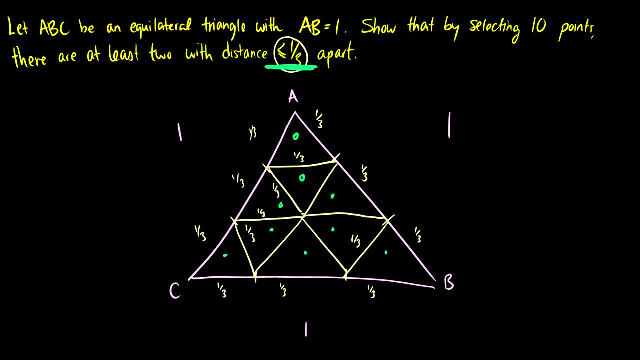 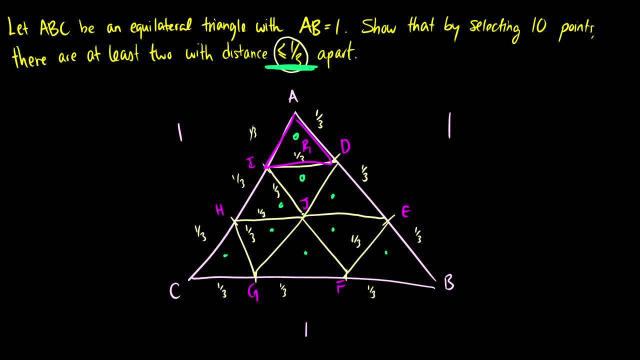 Using these triangles, you want to create regions R1,, R2,, R3,, R4, and so on and so forth, So you can define the regions with these labels for I, J, D, D, J, E, J, E, F- and then, with your regions, you can specify: okay, all of these regions at most.